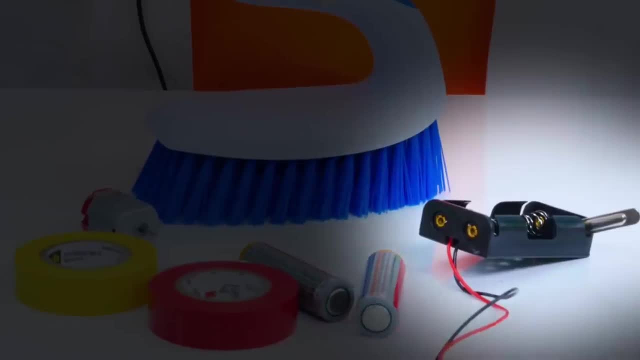 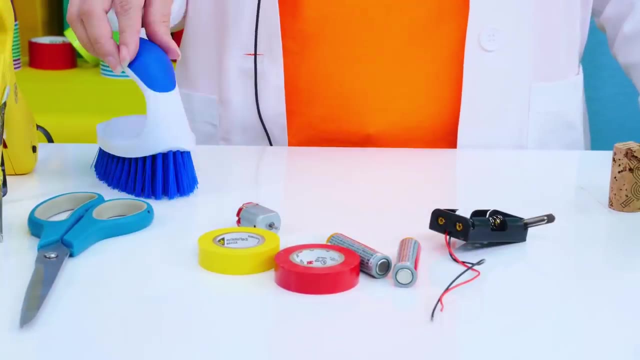 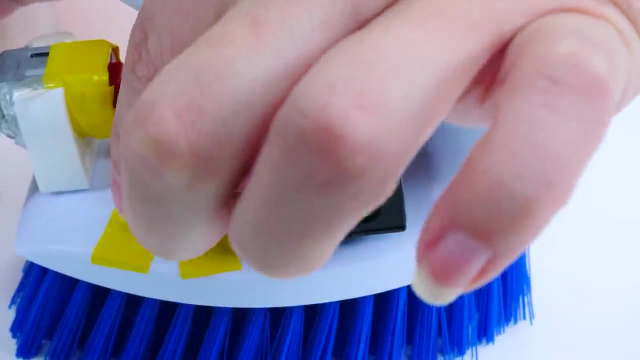 The first step in building our Brushybot is to wire the battery pack to the motor, creating a circuit. We happen to have these parts just lying around, but they can also be found online or at most hobby stores. Building these bots can be difficult and dangerous, so make sure that you ask an adult for help. 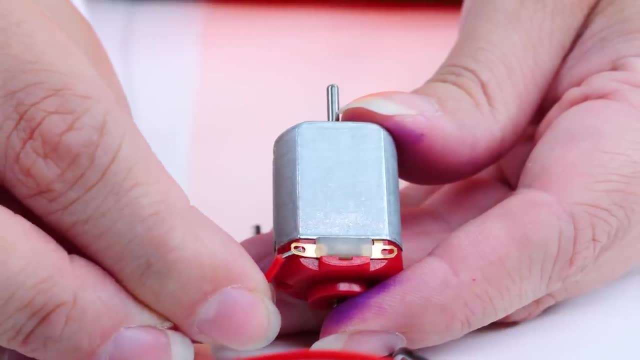 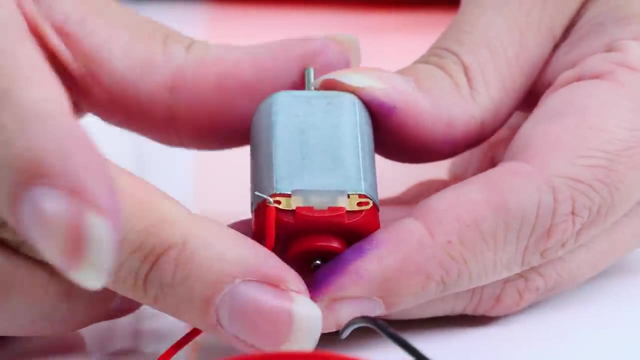 Wiring the motor is the most important step in powering our bots. We are going to connect the positive or red wire to the positive side of the motor and make sure that that is nice and secure. Then we are going to connect the black or negative wire to the negative side of the 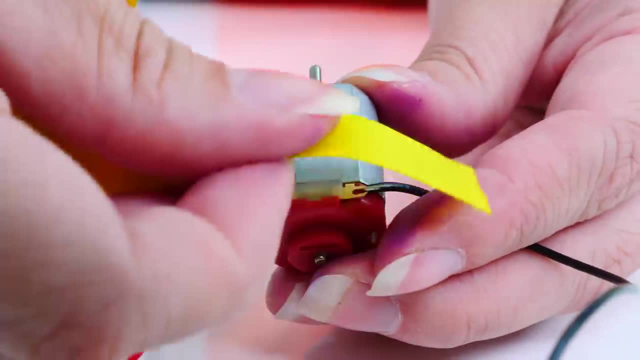 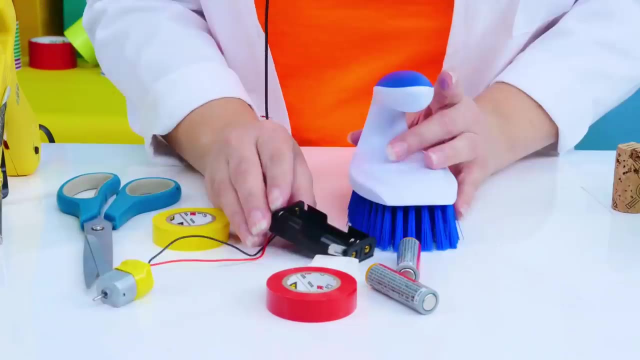 motor, just like that. Now we are going to wrap everything together with a piece of electrical tape to keep our connections nice and secure. First we are going to grab our brush. Next we are going to secure the battery pack and the motor bracket to the back of the brush. 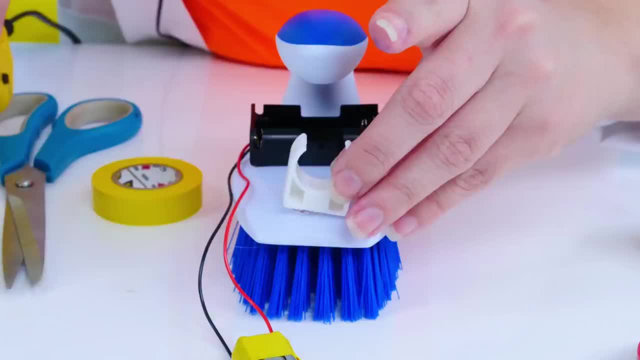 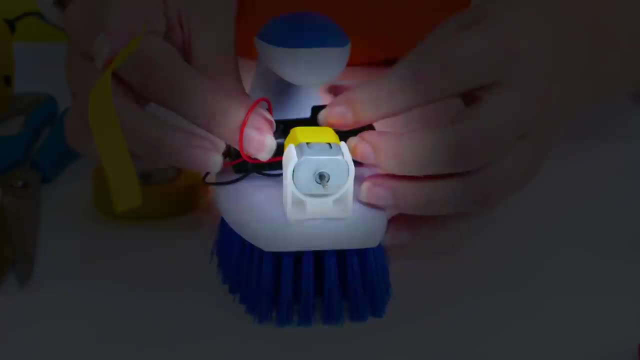 using hot glue. Once again, make sure to ask an adult for help, especially when using things like hot glue. Now I am using electrical tape to secure the battery pack and the motor bracket to the back of the brush using hot glue. Next we are going to secure the extra wires so that they don't get caught up under the 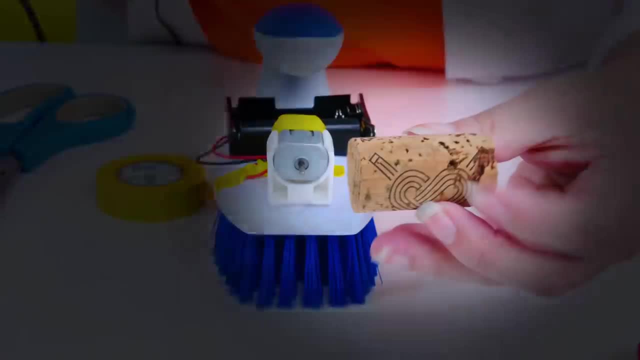 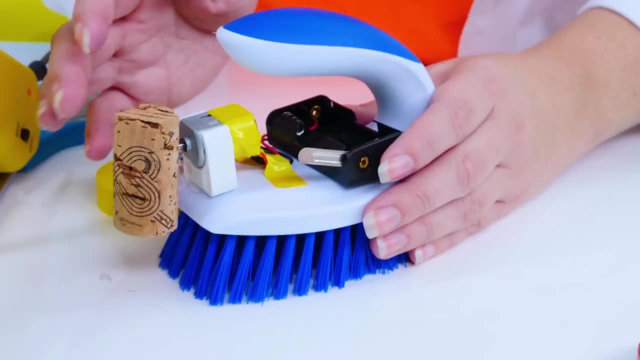 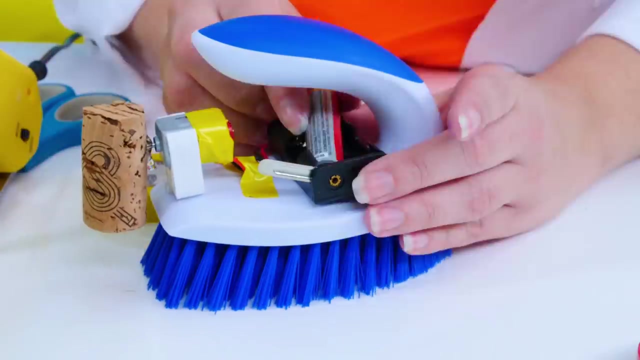 brush or in the motor. Now we are going to hot glue our cork to the post on the motor. It is important that the cork is attached off balance or lopsided so that when it rotates it creates vibration. This vibration is going to make our bot move. 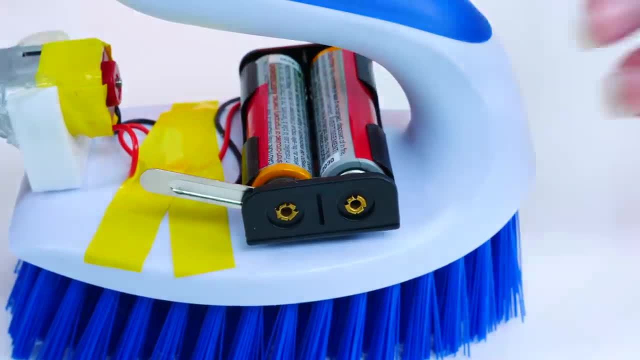 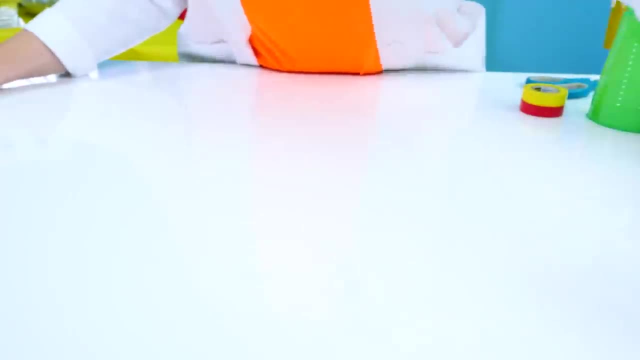 All that's left now is to add batteries. Now that we have everything built, all that's left is to flip this switch and complete the job. Let's see if we can do it. Woohoo, Look at him, go, Whoa. 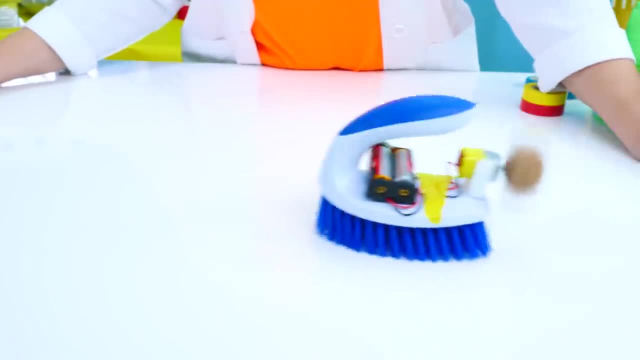 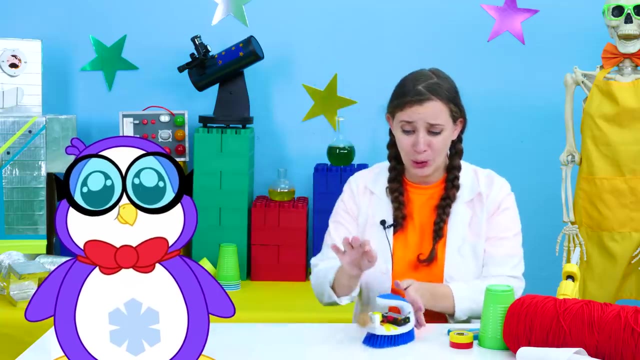 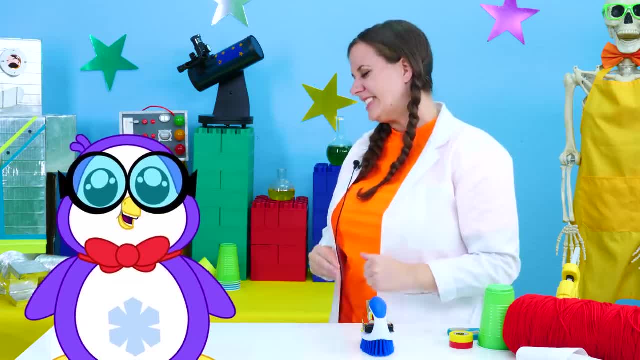 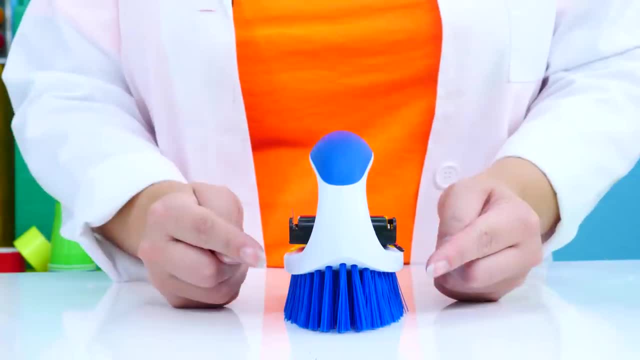 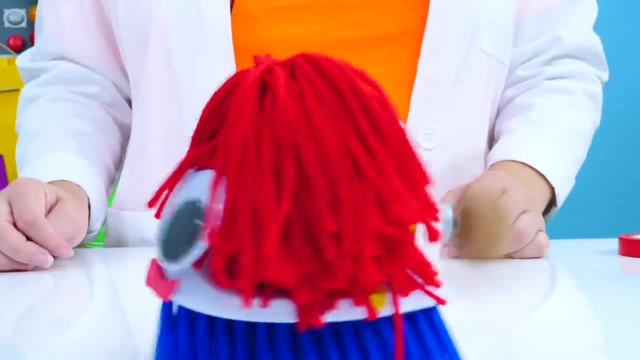 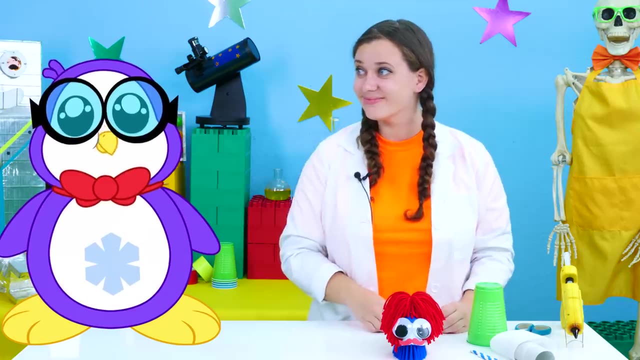 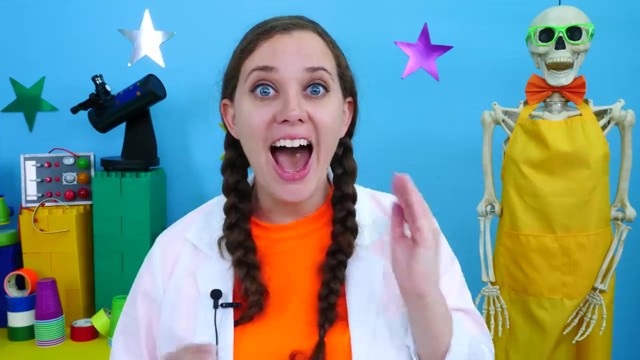 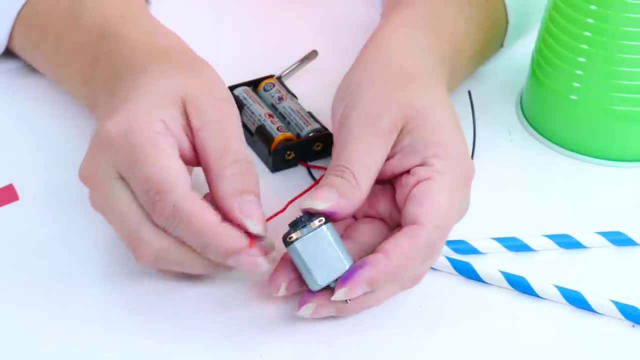 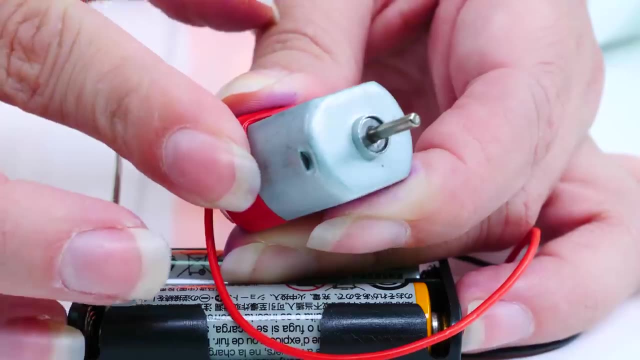 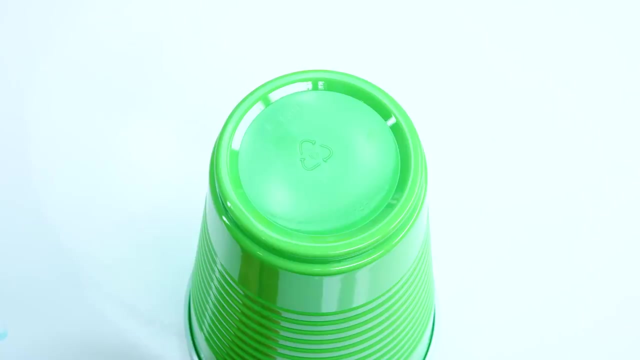 Oops. So, just like the other bot, we're going to start by connecting our positive wire and negative wire. there we go. that looks good and secure. let's test it out. sounds good. next we're gonna cut a hole in the top. make sure you ask an adult for help. now we're 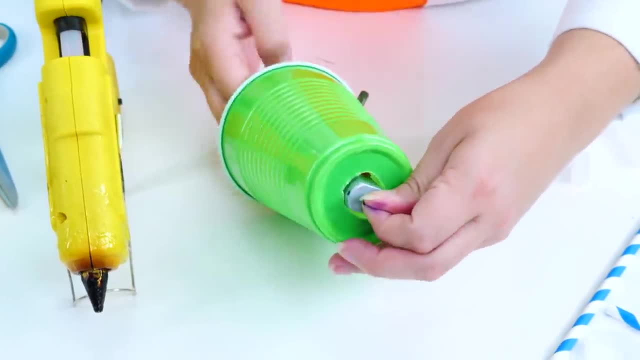 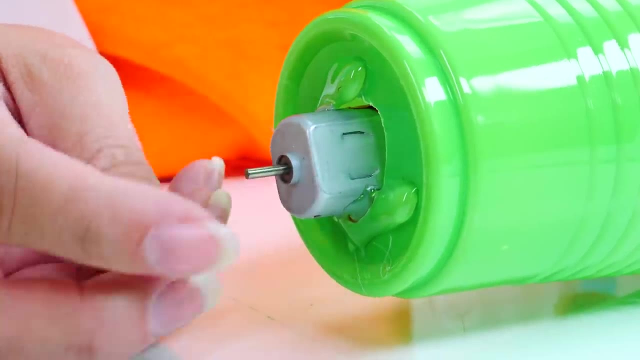 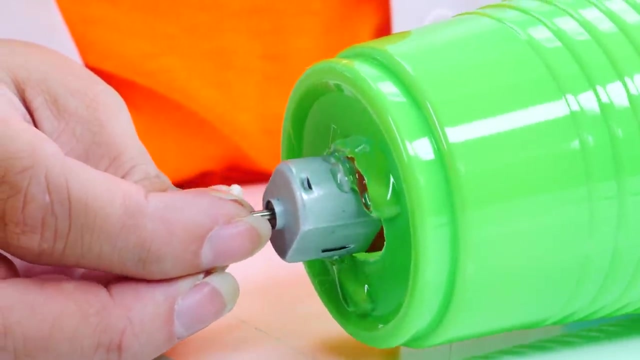 gonna attach our motor and our battery pack. so, starting with the motor, you have to be very careful as we glue this into place. the glue might take a while to dry, so we have to be very careful not to burn ourself and we need to make sure the motor sits in very straight. now we're going to 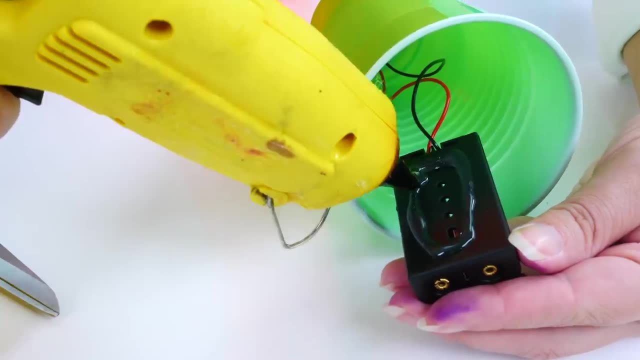 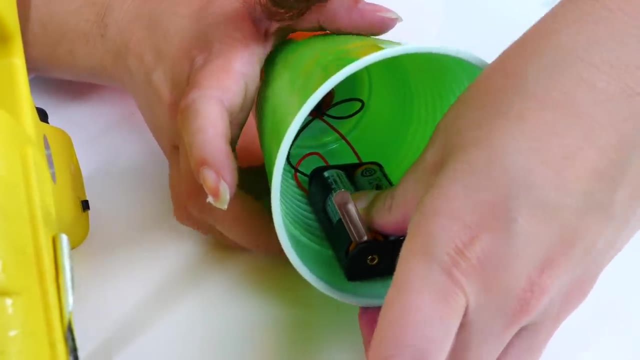 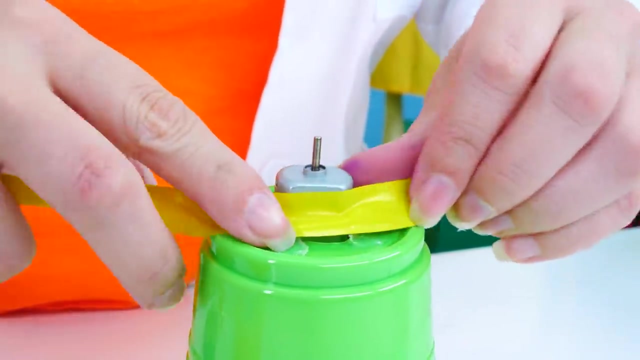 glue our battery pack in place. gotta use plenty of glue so that it sticks really well. let's put it right here where we can still turn on our lever. there we go. now i'm going to secure the motor extra, extra, extra with some tape. plus, it adds some fun color. so for our counterbalance we're going to 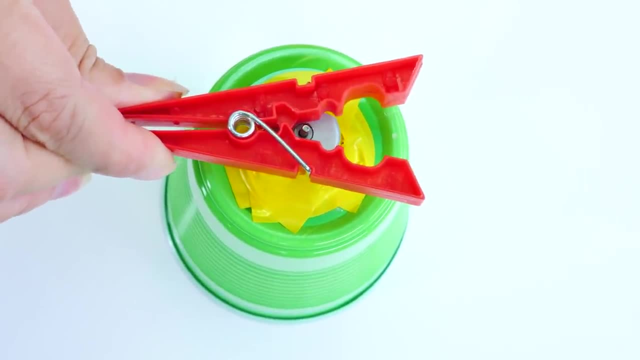 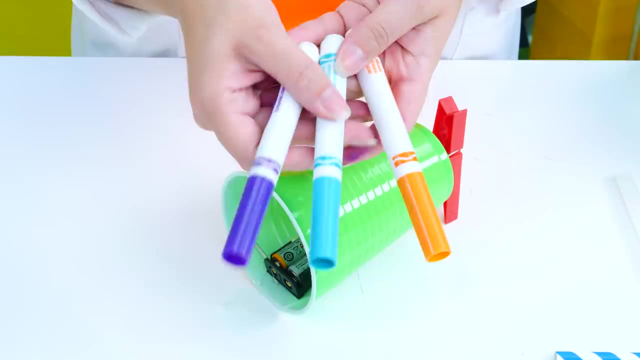 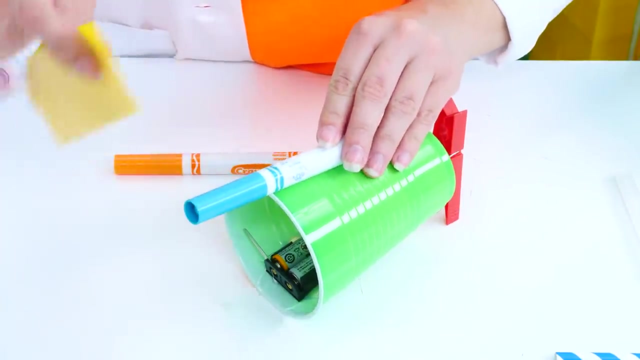 use this motor to secure the motor. so what we're doing is we're going to put a little bit of tape clothespin and clip it just like that. Ryan found us three markers. we've got orange, blue and purple, so we are going to tape them to our cup. Let's do the 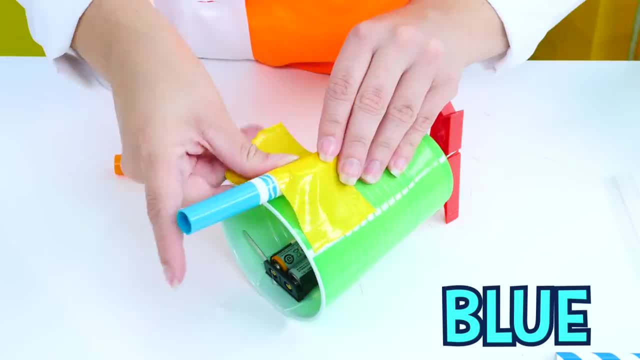 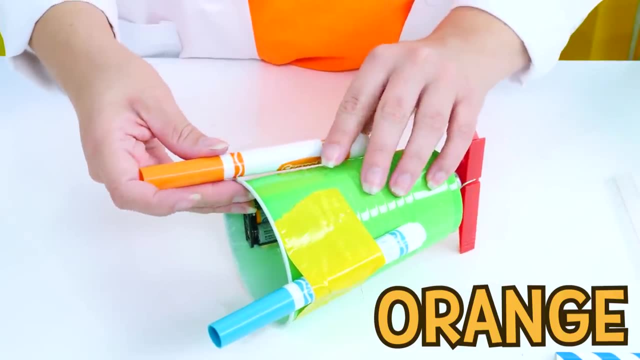 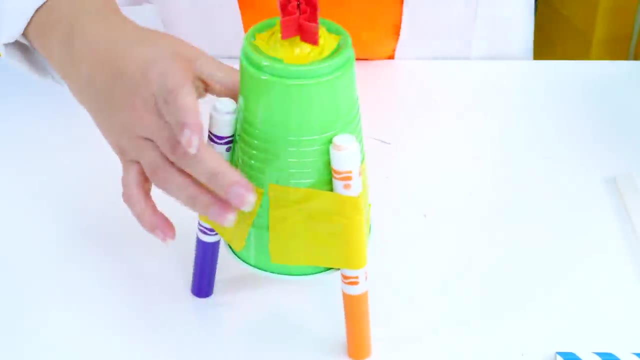 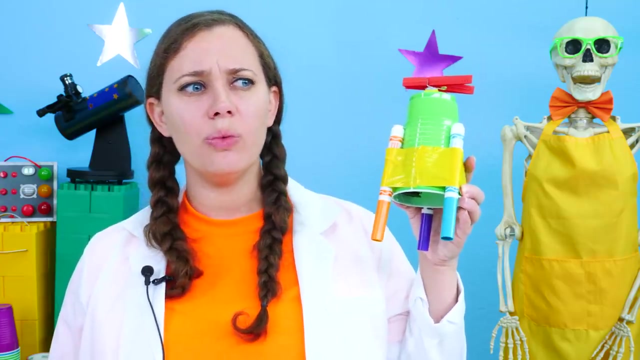 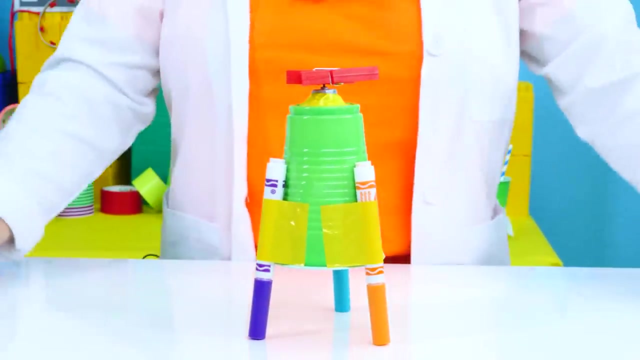 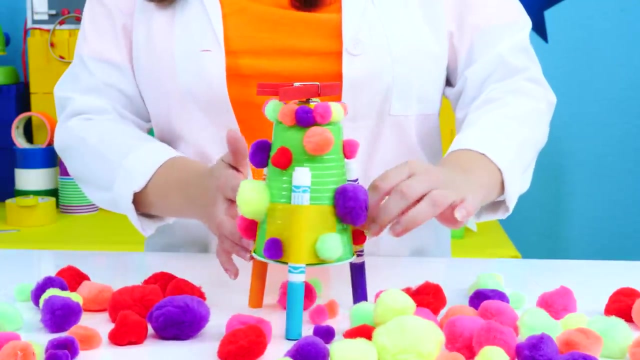 blue first. there we go, and then we're gonna do orange, and then the last one is gonna be purple. there we go, and ready to draw, I might add a few more finishing touches, And now we decorate. Ta-da, Look at all that color. Alrighty Bree, I laid out some paper for us to color on. 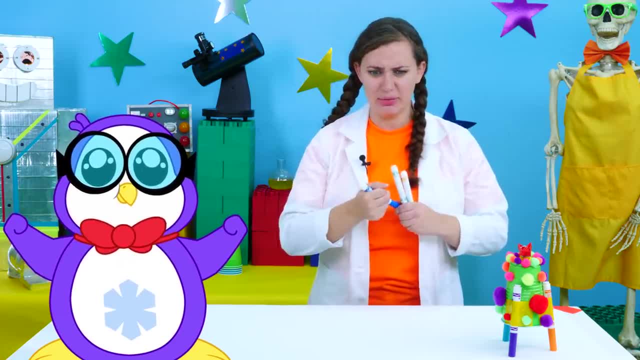 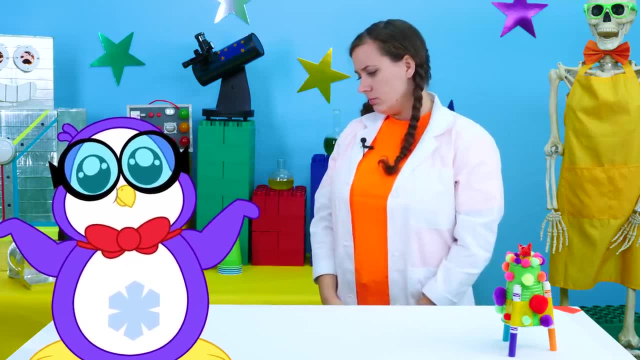 Coloring. Good thing, I go everywhere with my colors. I think I'm gonna start with maybe a house, and Oh wait, sorry, Bree, not for us for the bot to color on. Okay, well, I guess, I mean, this guy does look pretty cool. 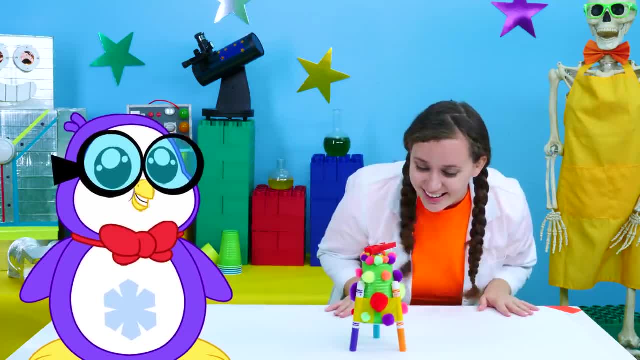 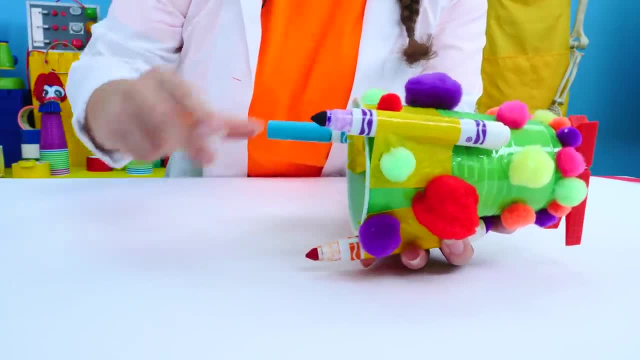 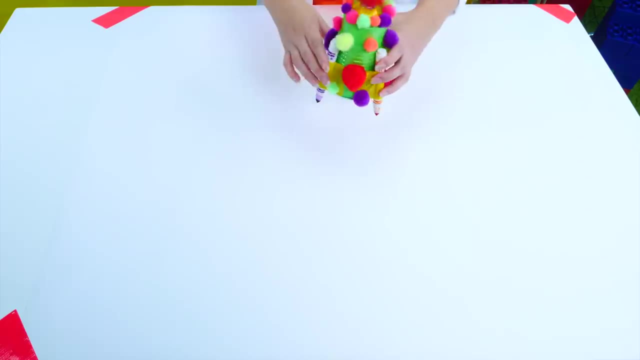 and I'm excited to see what kind of picture he makes- Hopefully some purple. First thing we have to do to start coloring is take off the caps. There we go. Ooh, look at those colors. Now we just have to flip it on. 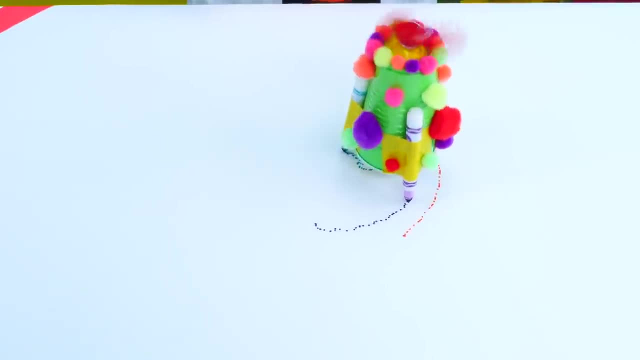 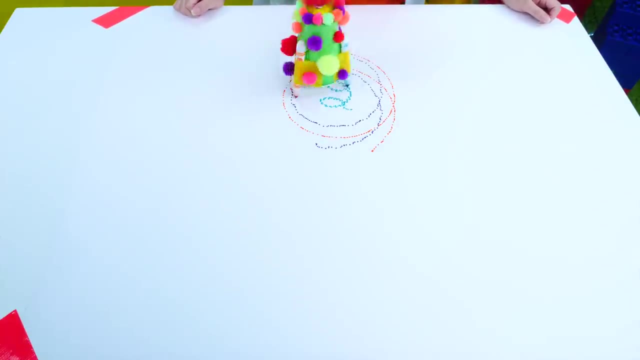 And now we draw Whoa, Whoa, fancy coloring butt, It's making circles. Oh no, he's falling off the table. Let's see, I think we need some more color here. Perfect Whoa. look at these circles it's making. 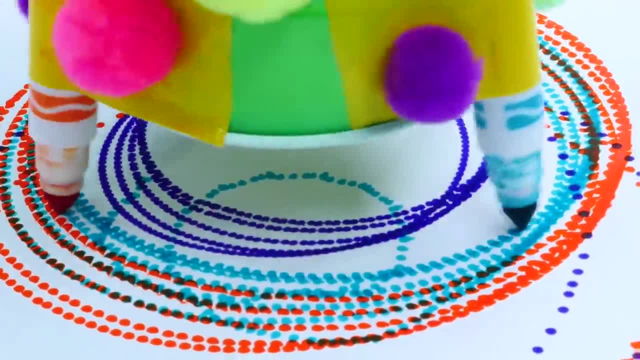 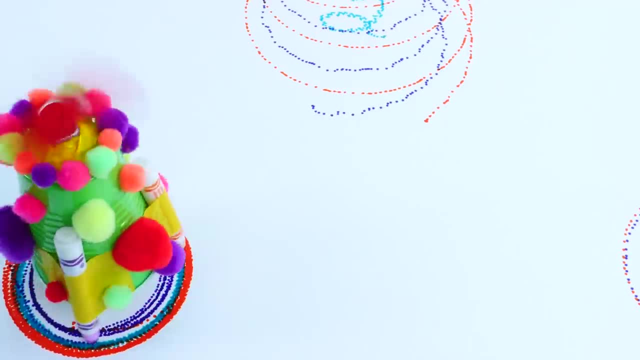 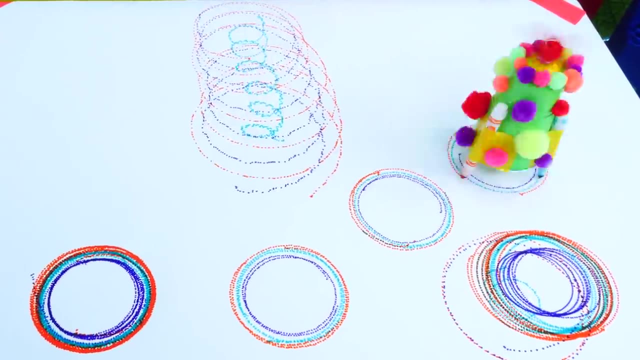 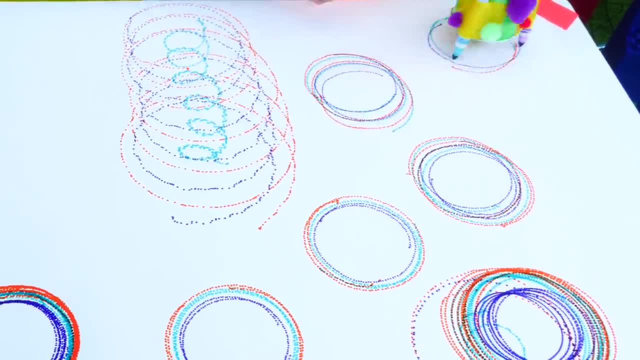 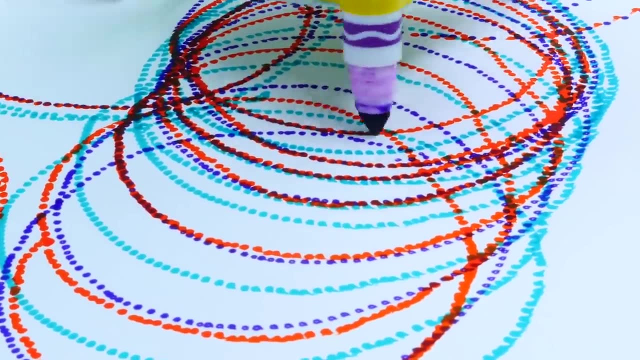 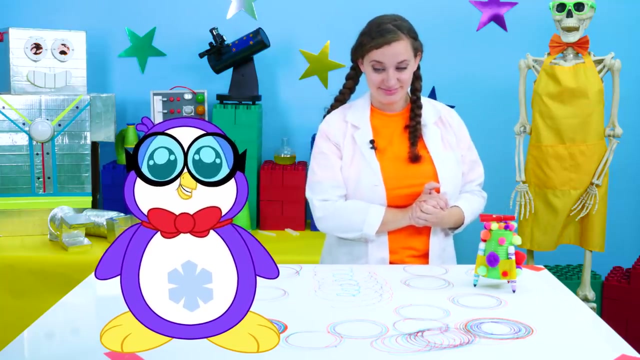 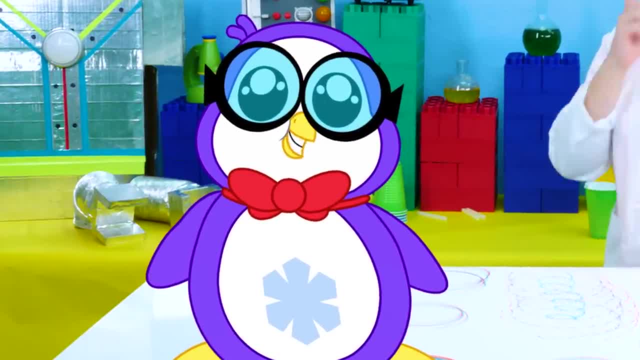 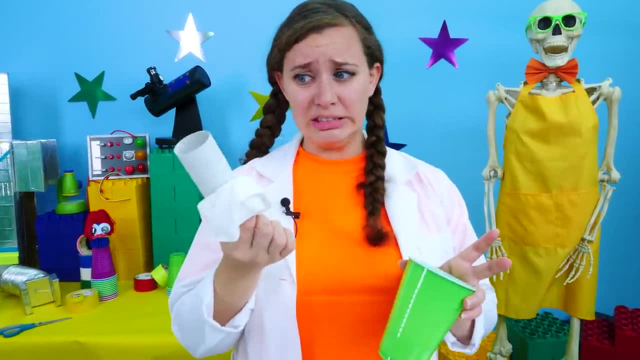 But can we make one more butt Bree? Well, we do have some straws. We do have some straws. We do have some straws And some toilet paper. Perfect, That'll be great for our next butt, If you say so. 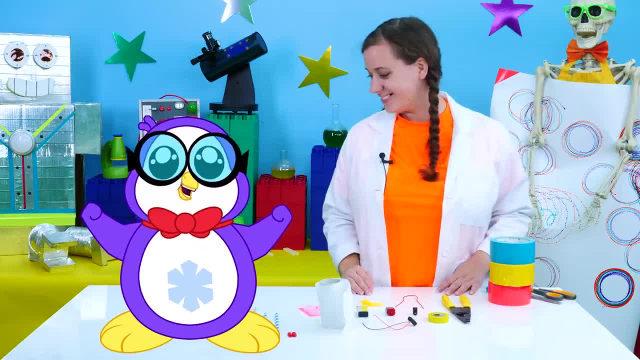 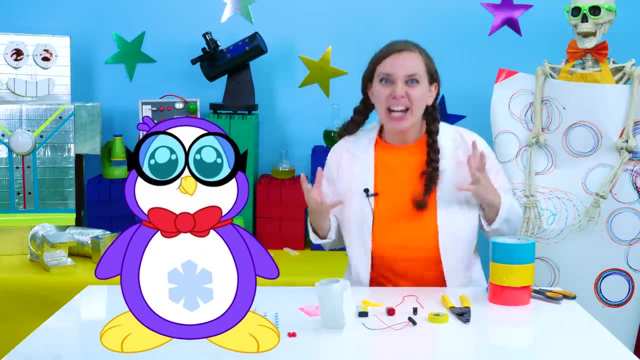 Okay, Bree, we have all our materials. Let's make a race car butt. Well, if you're asking me, my first answer is always the same: Let's decorate. First thing we have to do is fix this toilet paper roll. 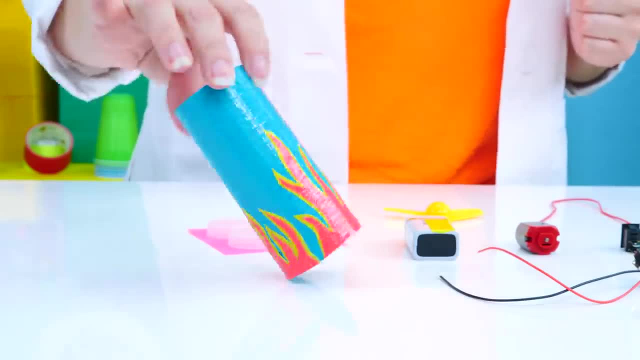 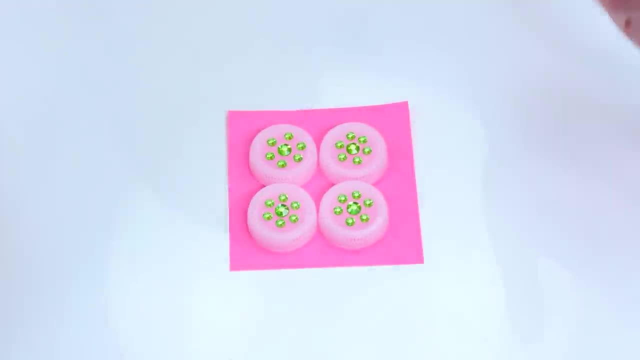 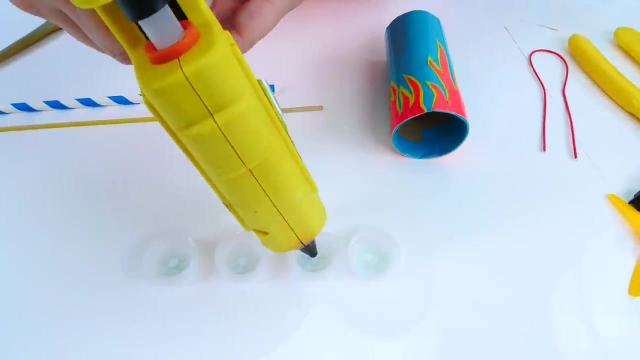 Now that looks like a race car. Now that looks like a race car. Now that looks like a race car Next up, these wheels need some bling There Now. look at that, All ready to go. Now we're gonna give this race car some wheels. 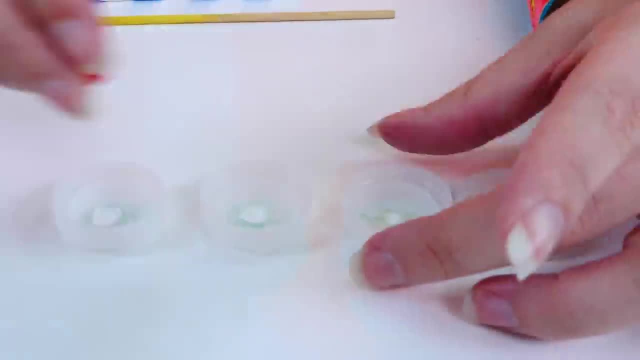 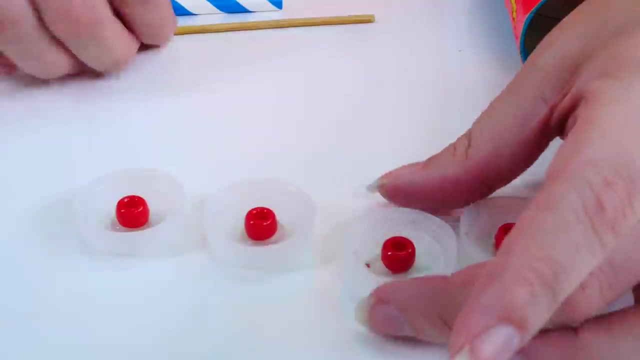 First thing we're gonna do is assemble our axles. Now we're gonna use these beads and glue them in the center of each wheel. This is gonna hold our axle in place. Now our axle is actually gonna be made out of the sticks and the straws. 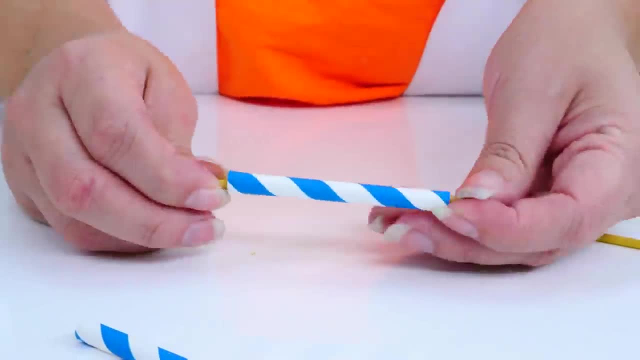 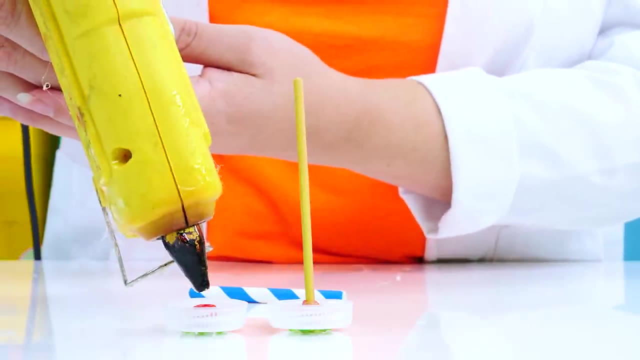 We need to cut the axles one size and the straws just a little bit shorter. This is going to allow for our wheels to roll. Now that we have everything cut to size, all that's left is to glue it all in place and put it underneath our car. 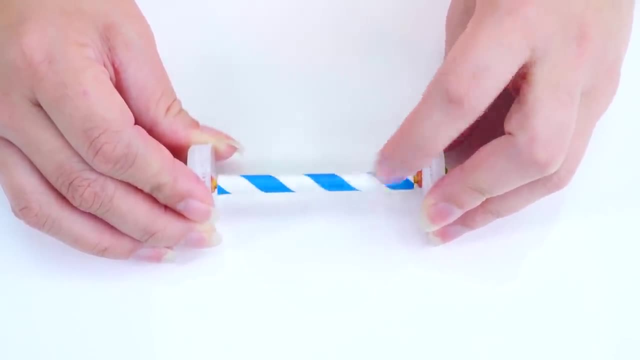 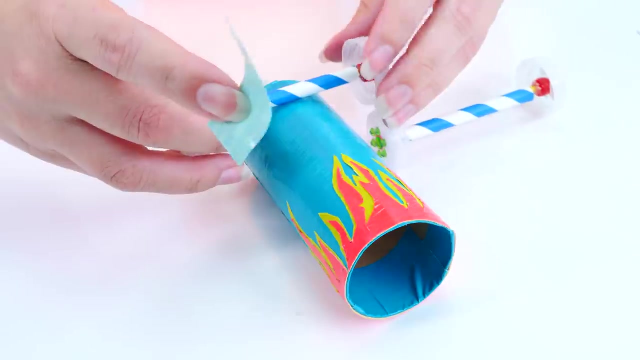 Once everything is dry, the straws should spin like this. Now, all we gotta do is build a second axle and, once that's dry, put it under our car. All right, Now we're gonna stick it to the bottom of our car. 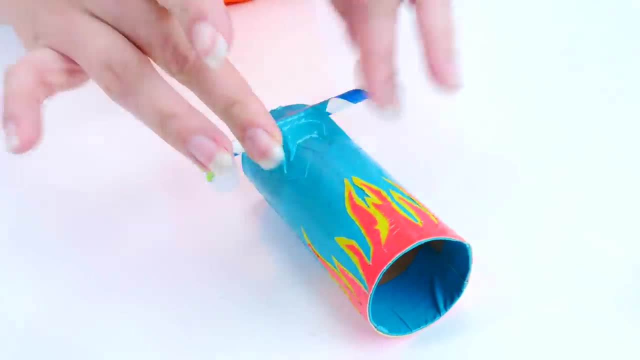 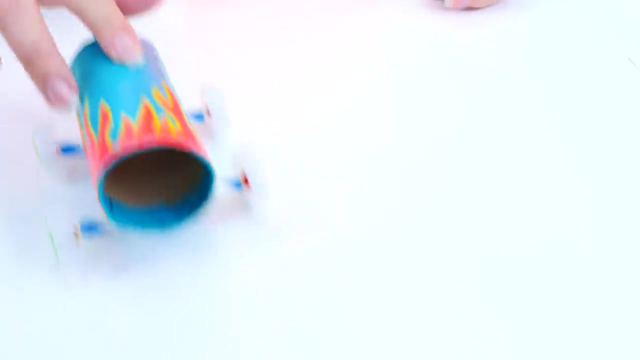 Now we're gonna stick it to the bottom side of our car using duct tape. We have to be really, really careful to make sure we stick the axles on straight and in the middle so that our car will go straight. Now is the tricky part. 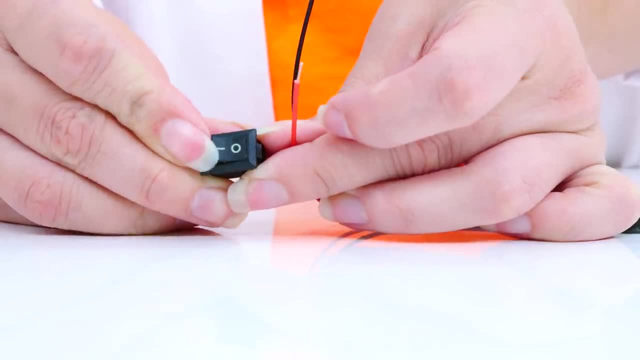 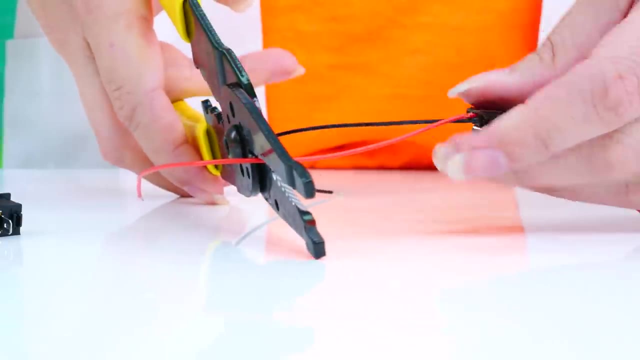 We are going to use this on-off switch to turn our car on and off, So, in order to do that, the first step we're gonna have to do is to lengthen our positive wire, because it's too short to run all the way through the car to the back. 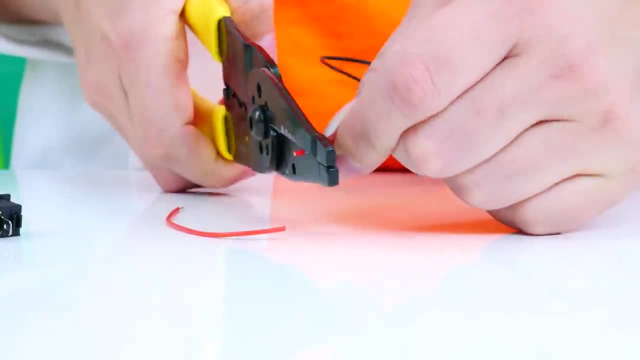 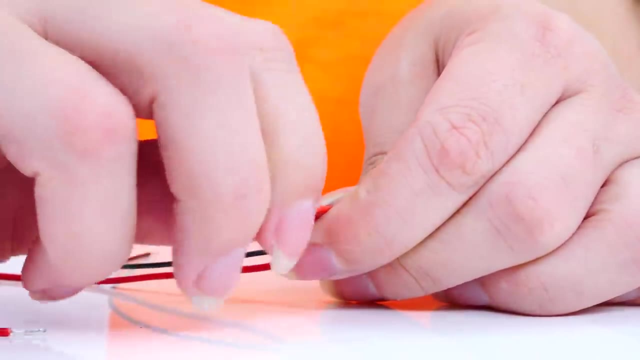 To do this, we're gonna cut our wire in half and then, using wire strippers, we're going to take the coating off of both sides so that we can thread them together. Now we're going to take the two ends of exposed wire. 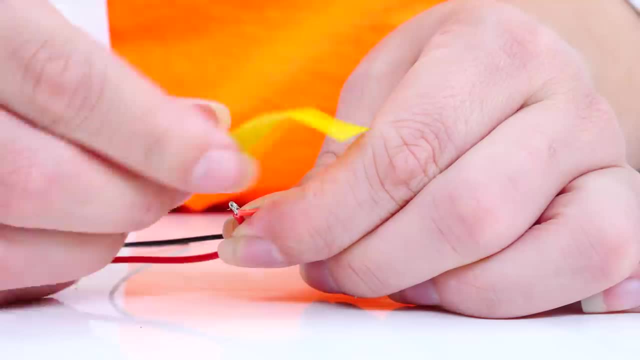 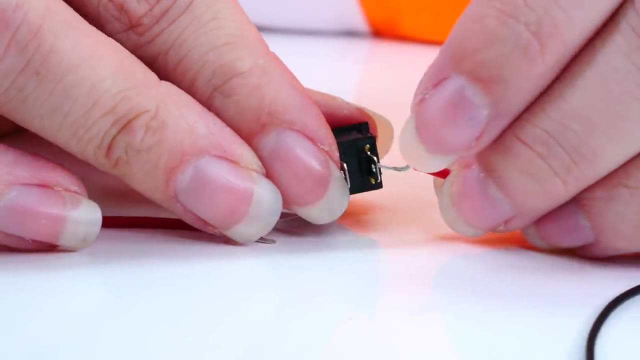 and we are gonna twist and twist and twist nice and tight and then cover it with tape for safety. Now that that is nice and secure, it's time to put in our switch. We're going to take two positive sides and thread it through each side of the switch. 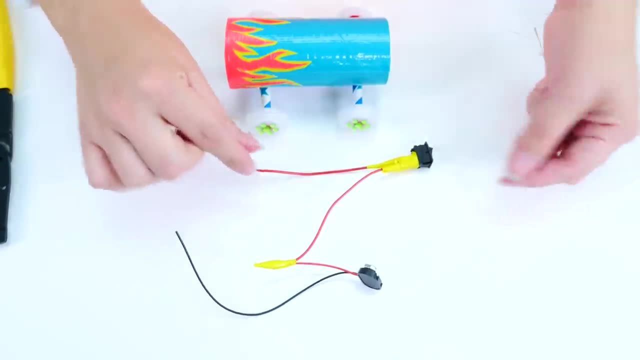 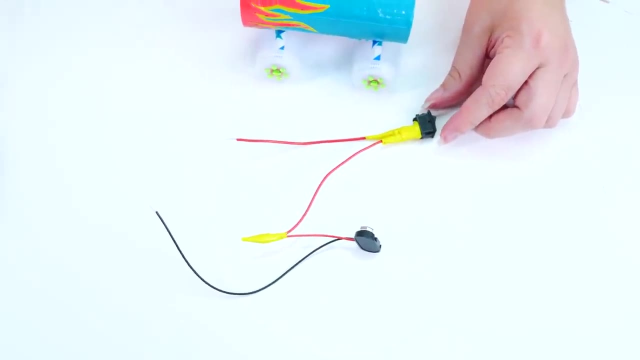 We're gonna bend over the wire to make little loops and then secure that with more tape. Now that we have our switch in place and that looks nice and secure, it's time to wire up the motor. We are gonna start by attaching the negative side. 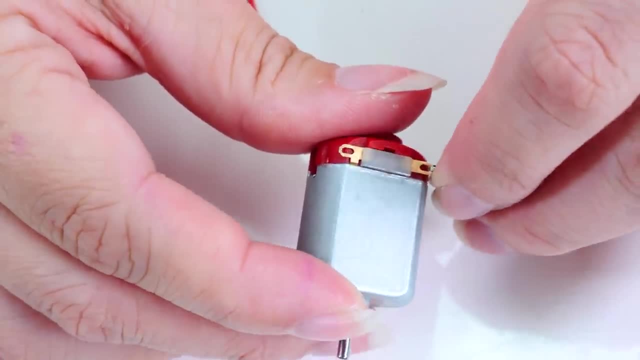 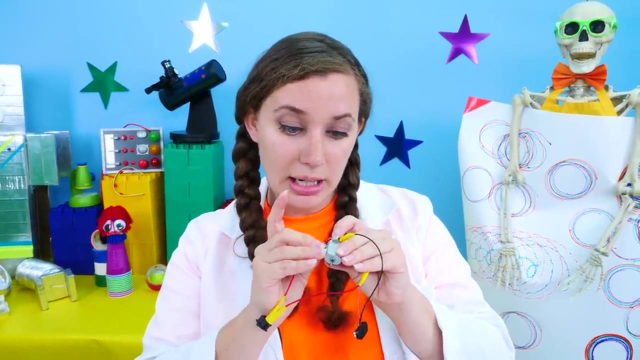 to the negative side bending over the wire. so it's nice and secure. Now that we're done taping the negative side, let's connect and tape up our positive side, And there we go. hopefully we can get this nice and tight with some tape. 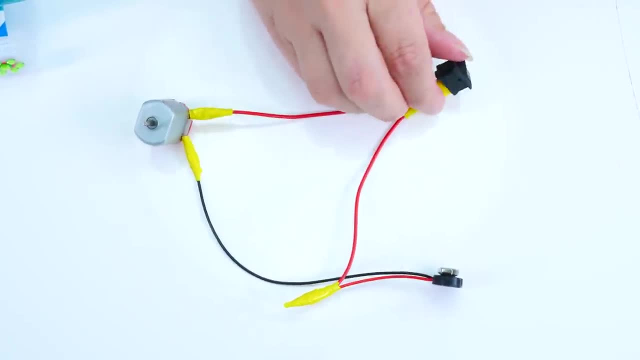 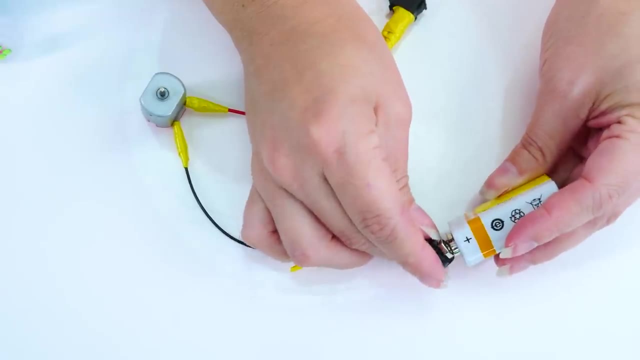 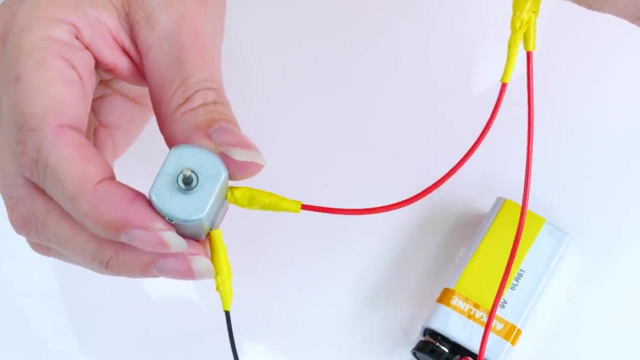 So now that we have our circuit connected with our motor, our on and off switch and our battery pack, we need power aka battery. So if we connect this, then we hit our on-off switch. it turns on like that: 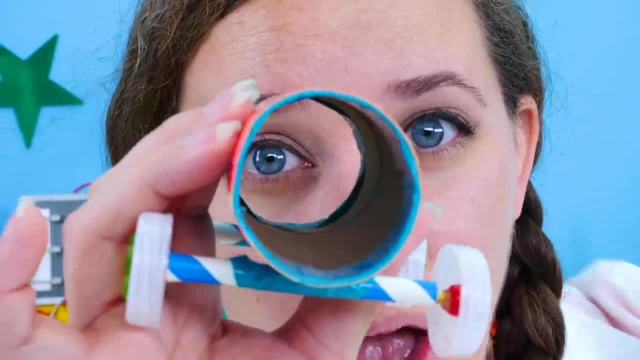 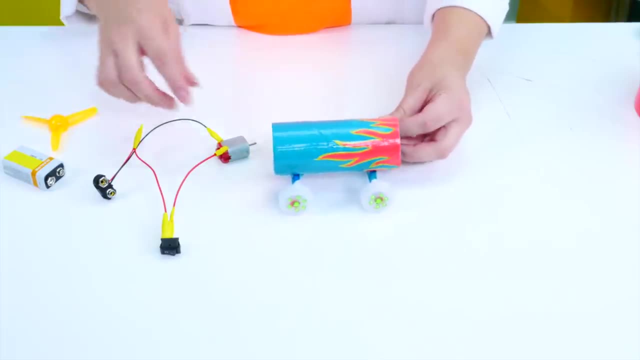 Next step is to install our finished circuit inside of our race car. We are gonna put it in here So that way it can go zoom. The first step is making sure our motor is attached in the front with enough space for our propeller. 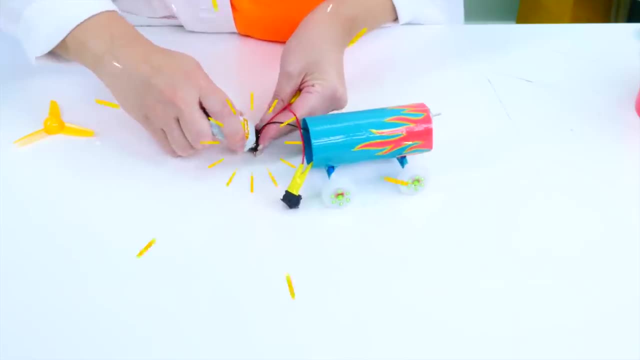 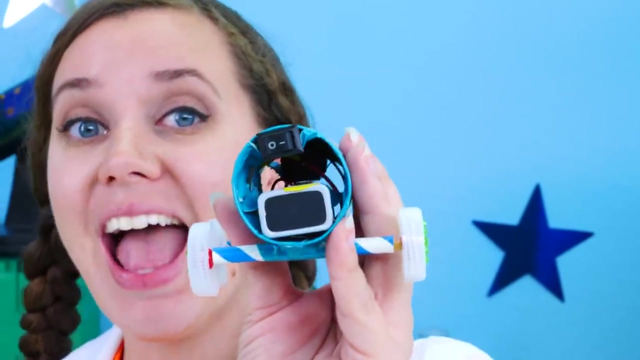 Now that that's in place, we need to make sure our battery pack is nice and secure in the back. All that's left is to attach the switch. Ooh, now we have our circuit installed. I put the on-off switch in the back. 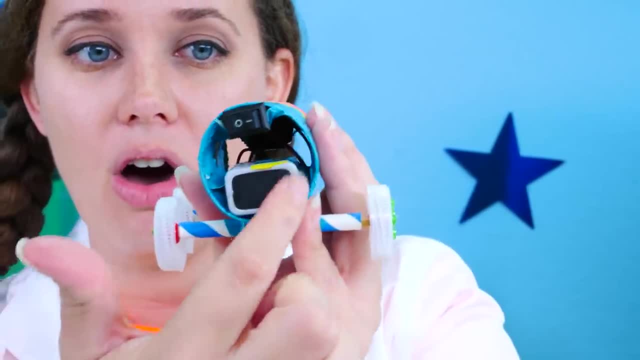 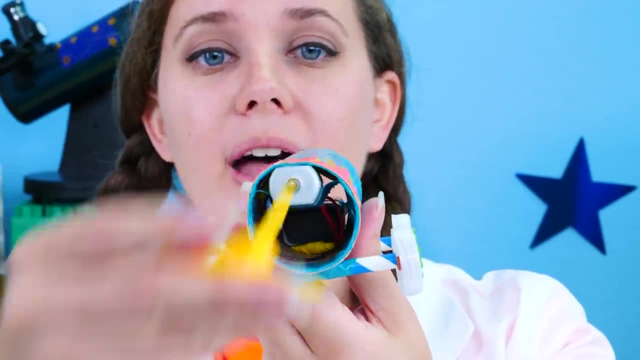 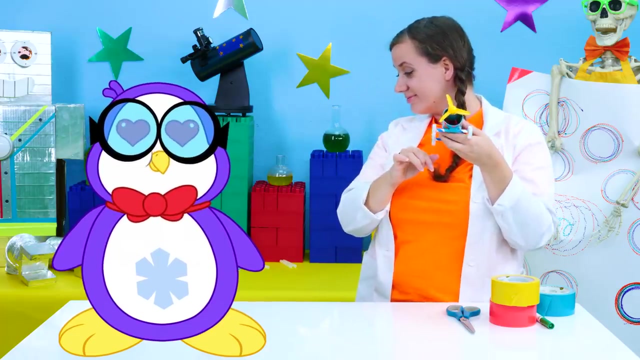 so it's easy to turn on and off. We've got the battery, all the cables and the motor up front. The last thing that we need to do is to put on our propeller And done. Ooh, let's go for a test drive. 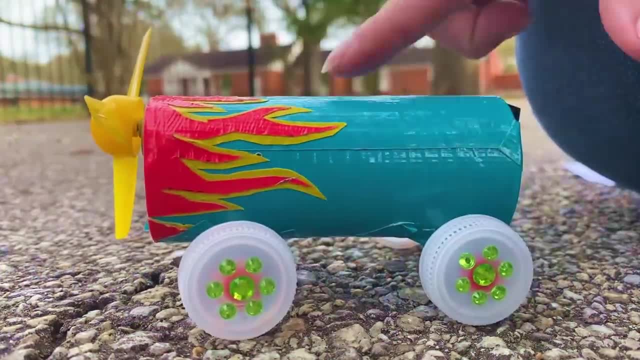 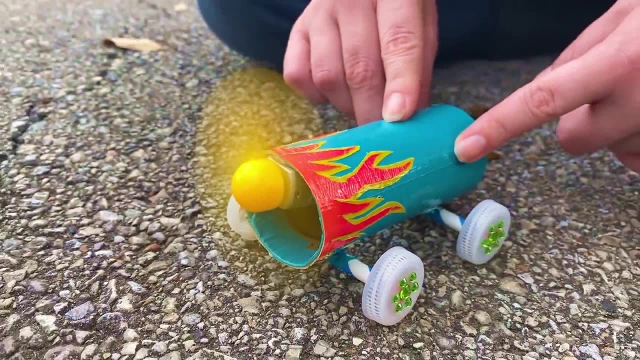 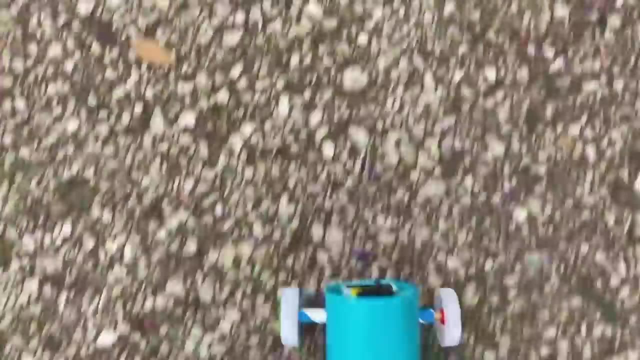 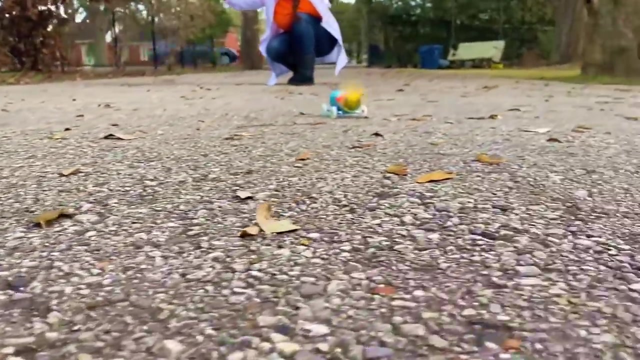 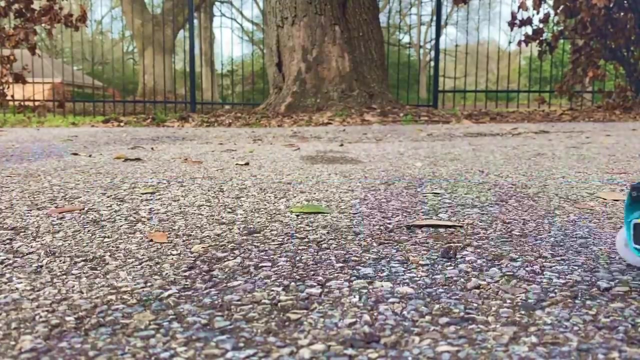 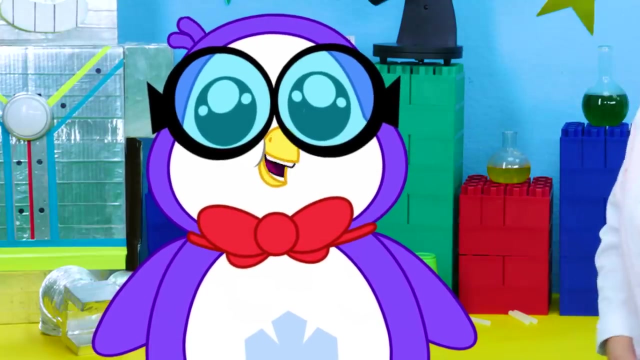 You heard the penguin. let's go Go, race car go. This spot is spectacular. That was so much fun. I think it's time we send these over to Ryan, As much as I would love to play with them. 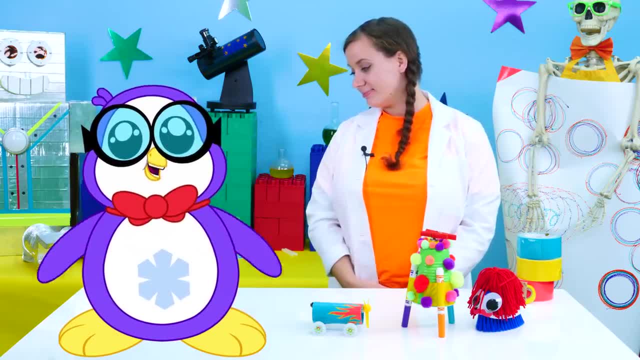 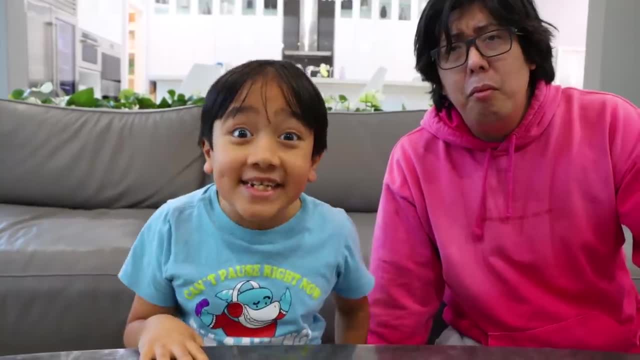 I think you're right, Teleporting the bots over to Ryan. Ha-ha, Oh, Oh, Bye bots. Hey Ryan, What are you doing? I'm waiting for Peck to send me his latest invention, Hey guys. 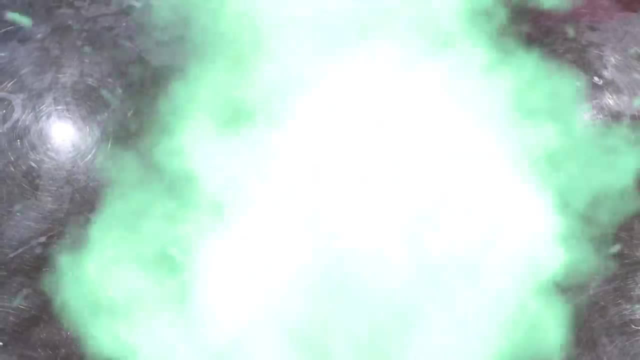 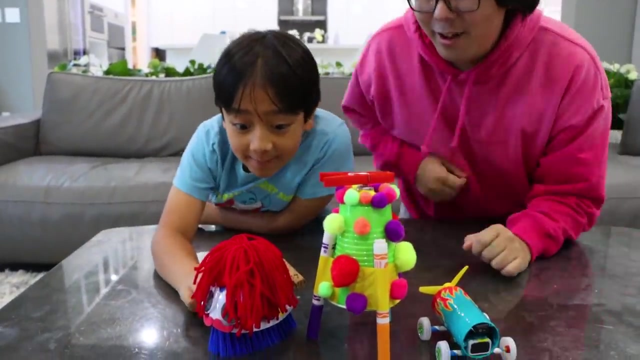 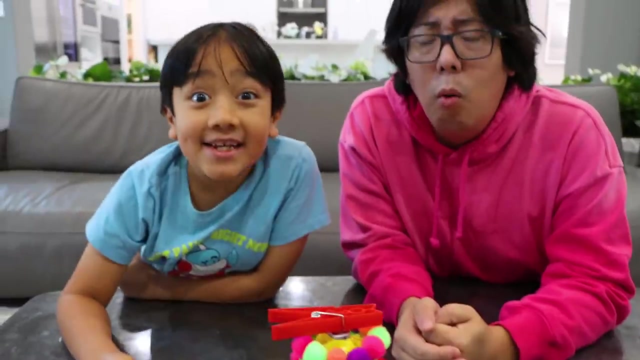 Oh hi, Peck, Is it ready? The bots are ready, Ta-da, Whoa, That's so cool. Wow, Peck, Amazing work. What are these? So I sent Peck a bunch of random stuff and he said he could make a robot with it. 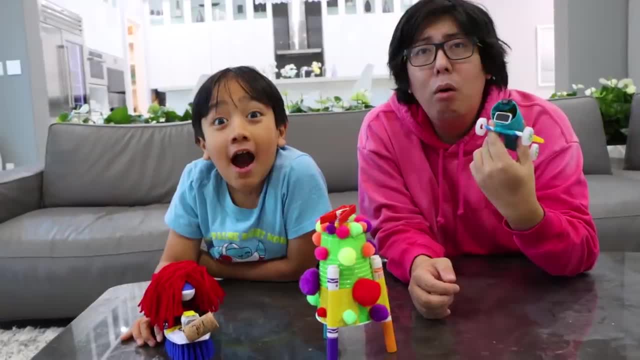 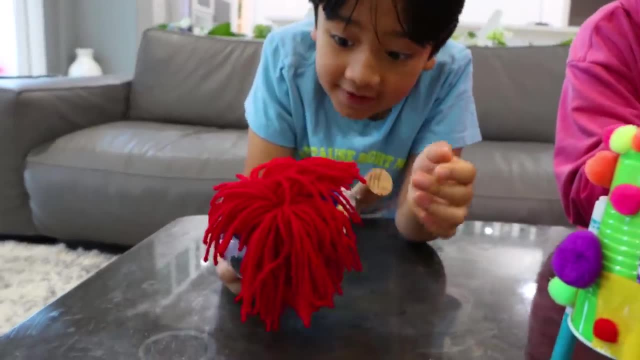 So these are robots. Yeah, Make sure to test them out. Have fun, Okay. Do you see a button, Ryan? I see a button over here. It's a lever. Let's see what it does. Whoa, Whoa. 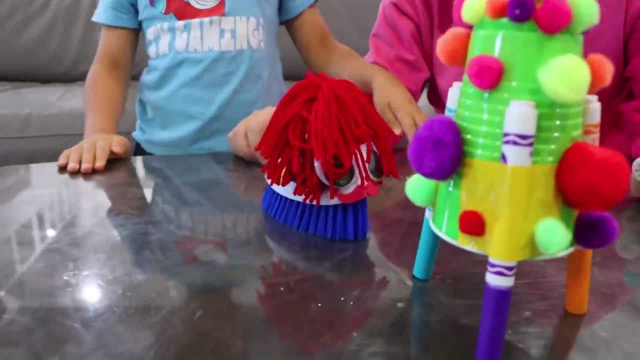 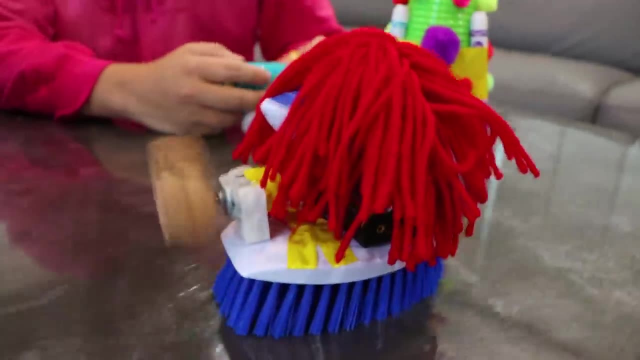 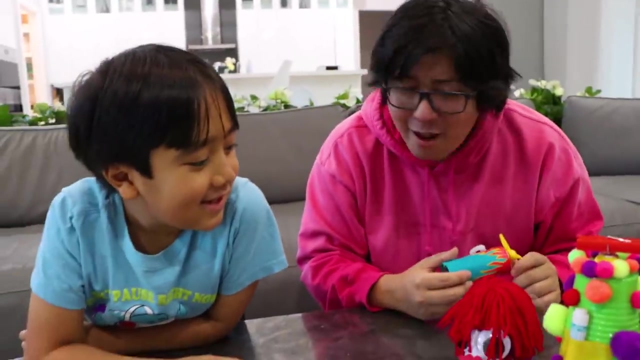 It's going backwards. It's cute- Backwards airplane. Where are you going? Where are you going? Oh, we should name him. He's so cute. Oh, it's like a pet Robo-Pet. What's his name? 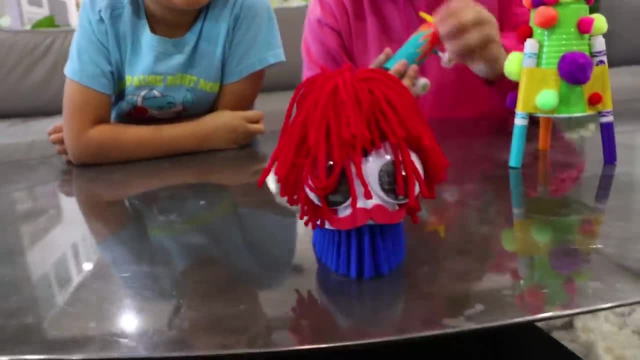 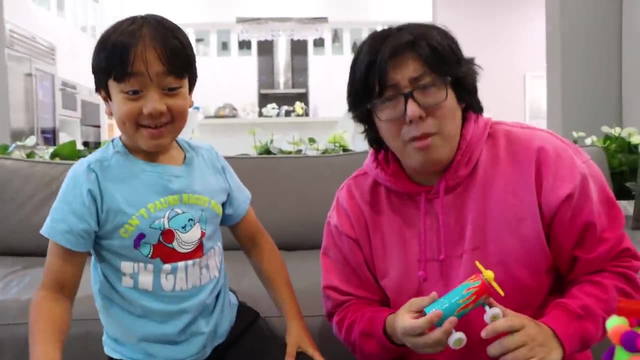 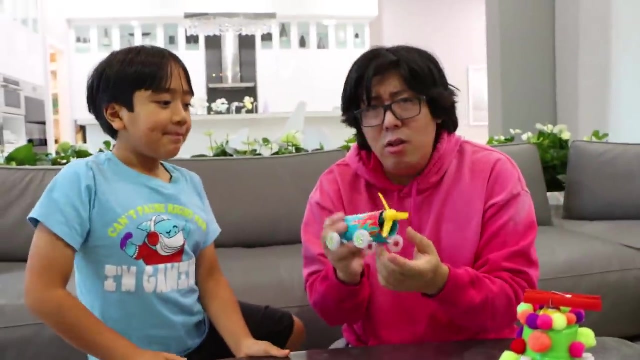 Uh, hmm, Maybe Bear-plane, Because it's like an airplane, but then it goes backwards. Bear-plane, Okay, Aw, so cute. Hi, Bear-plane, Okay, Oh, Okay, my turn. So this one. I found the switch right here. 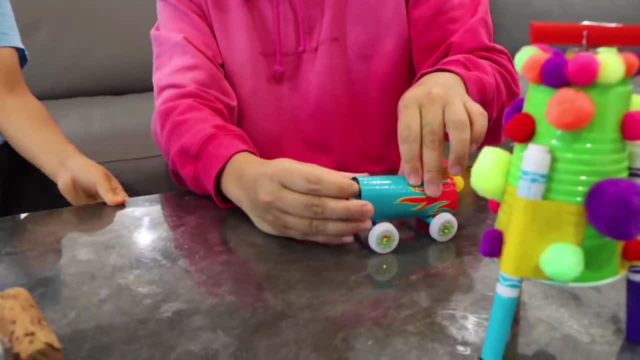 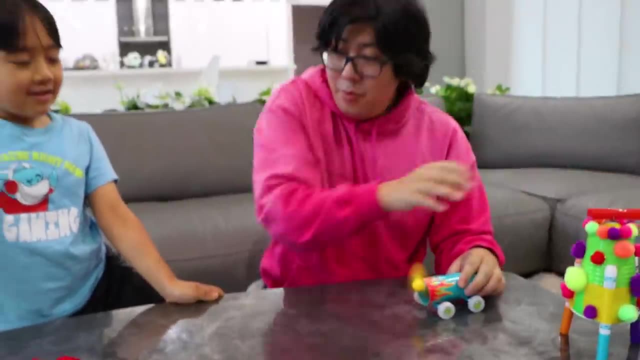 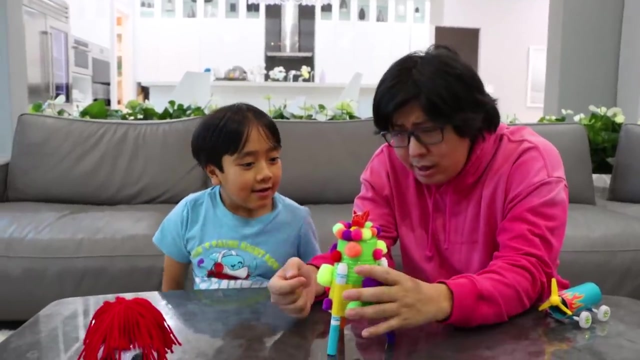 Let's see if it works. Whoa, Whoa, Whoa, Whoa. It moves, Whoa, Okay, ready, Yeah, Move your hand. Move your hand, Ready, Okay, go, Whoa, All right, just the last one. 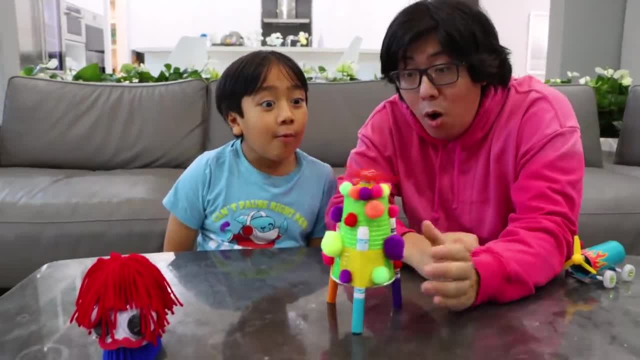 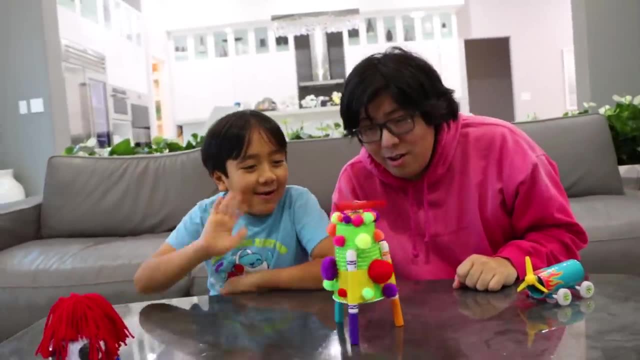 Let's see. Okay, Let me turn it on. Whoa, Whoa, It's spinning. Whoa, Whoa, Whoa, It's coming toward us. Oh, Hello, Hello. Don't forget that it can also draw too. 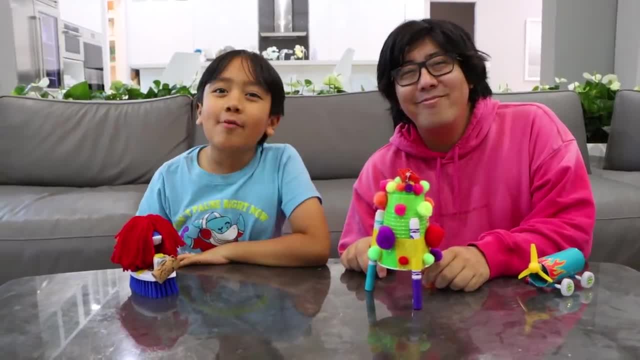 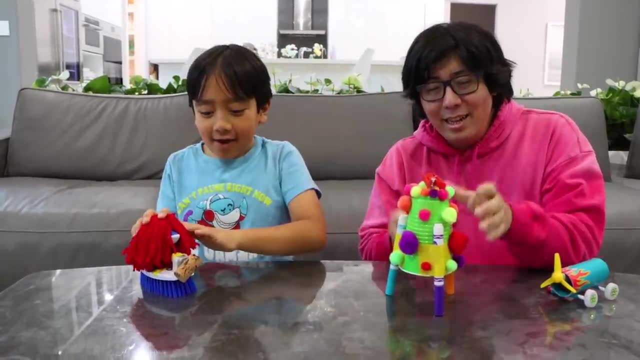 Yay colors. Thank you for watching our video. Thank you for watching our Making Robots with Everyday Household Objects video. Bye, Remember. always stay happy and rise up. Bye, Bye, All right, turn it on. Yay Whoa. 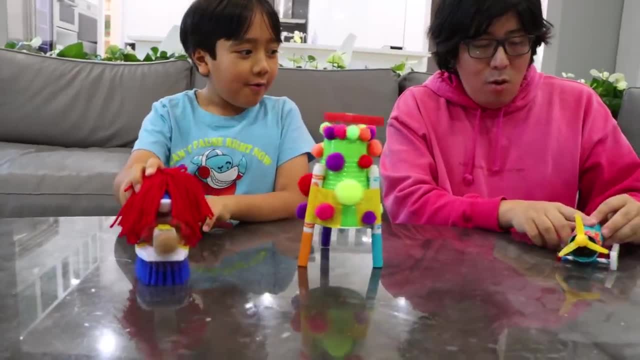 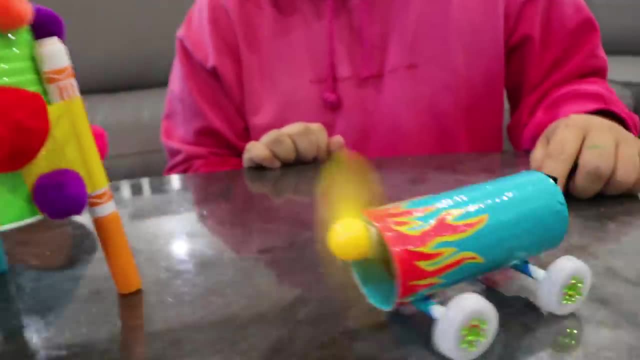